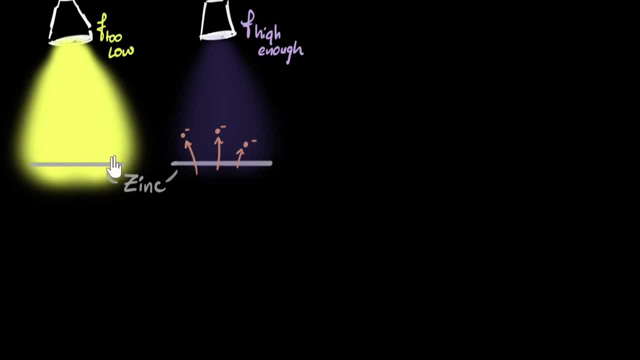 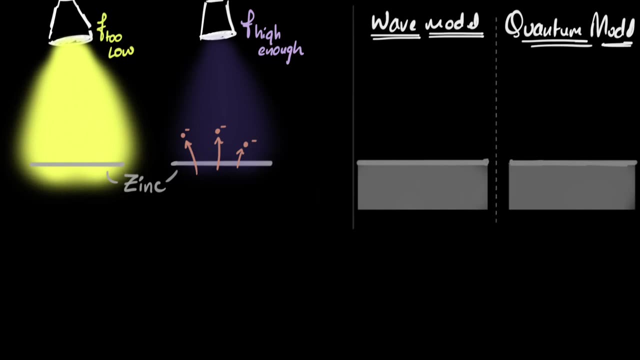 of photoelectric effect, as to why the brightness or the intensity doesn't matter, but it's the frequency that matters. So let's begin. So let's consider the wave model and the quantum model separately. Let's start with the wave model. Imagine this is our zinc metal. 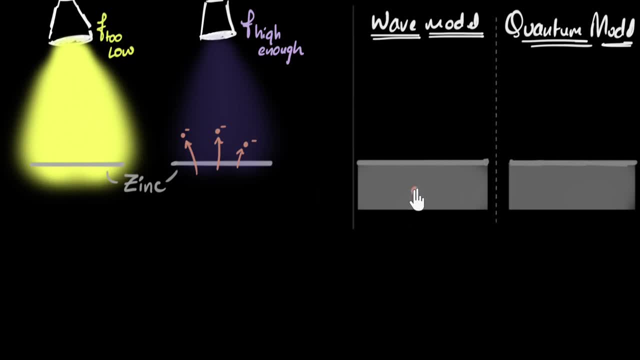 and here's an electron trapped inside the metal. Now, for it to escape, it needs to gain some energy. For simplicity, let's say it requires three units of energy. Now, according to the wave model, light is a wave and when you shine light it's a wave. 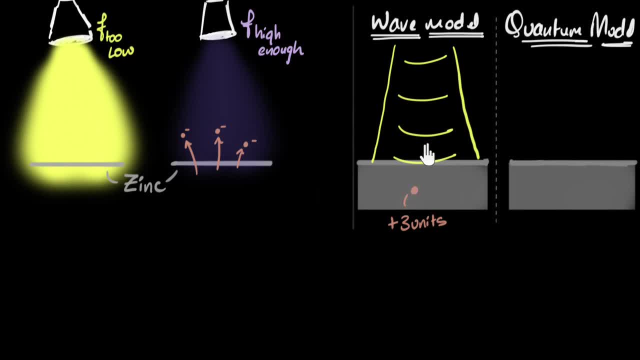 when you shine light, the electron starts absorbing the energy from this wave, and so the electron's energy will start increasing from whatever it is right now. It'll be at plus one plus two, and finally, once it increases beyond three, it has now enough energy. it escapes from that metal. 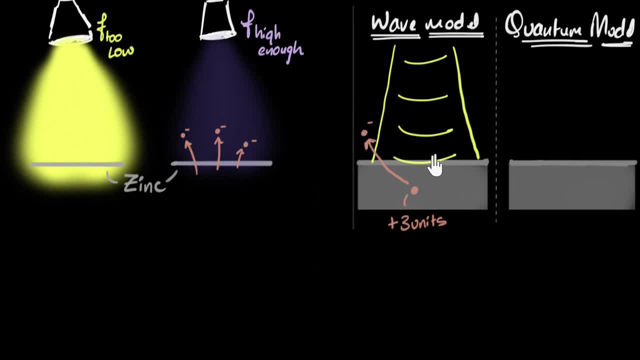 It's happy it goes. photoelectric effect And according to this model it doesn't. It doesn't matter what the frequency is, Any frequency light you shine, the electron must gain enough energy eventually and should just escape. And in fact, according to this model, 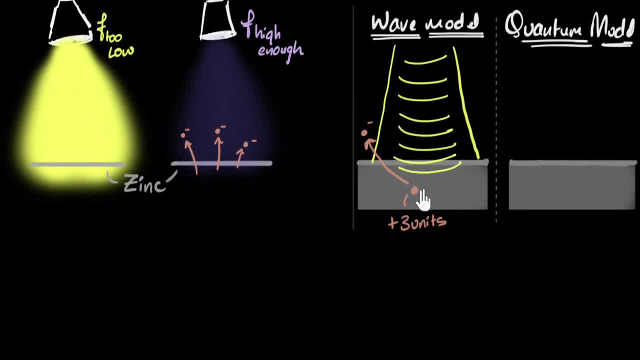 if you shine brighter light, the electron gains so much more energy and it should be able to escape much more easily, And therefore you should get more photoelectric effect over here, And that's why, according to wave model, it doesn't make sense. 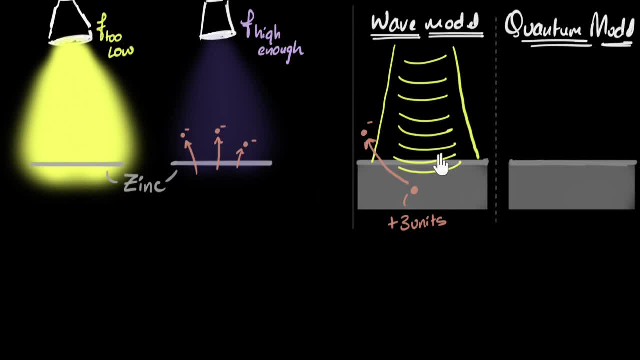 Why does the frequency matter and not the intensity? But now let's see what the quantum model says. The quantum model says, hey, light is not made of waves, it's made of photons. And we've explored this right, According to the quantum model. 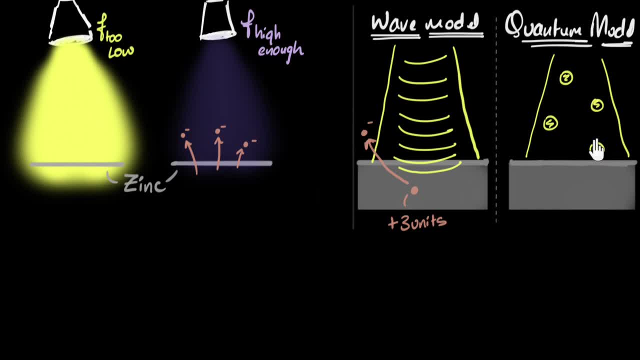 light is made of particles, what we call photons. Now what happens when an electron absorbs this photon? Same electron again. even this one needs three units of energy. Let's take some numbers. Let's say the energy of this photon is five units. 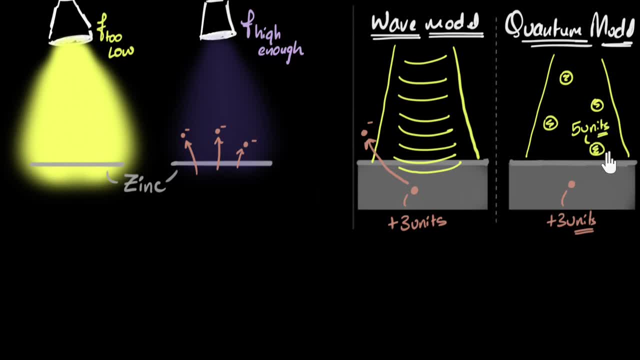 It has five units of energy. It's a packet that contains five units of energy. Now, when this electron absorbs this photon, it absorbs that five units instantly. What this means is that the energy of the electron instantly jumps plus five. And try to understand what that means. 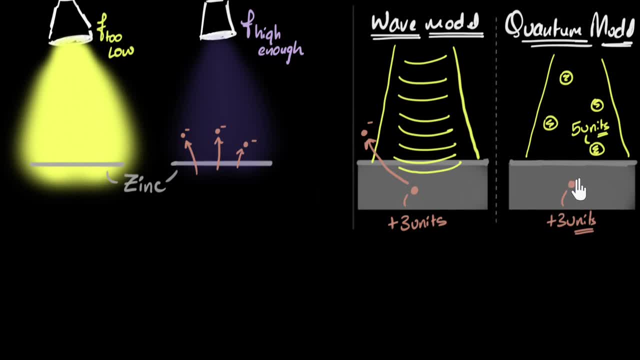 It doesn't go plus one, plus two, plus three, plus four and then plus five. It instantly goes plus five. It's kind of like your car going from zero to 100 kilometers per hour directly without going through plus 10, plus. 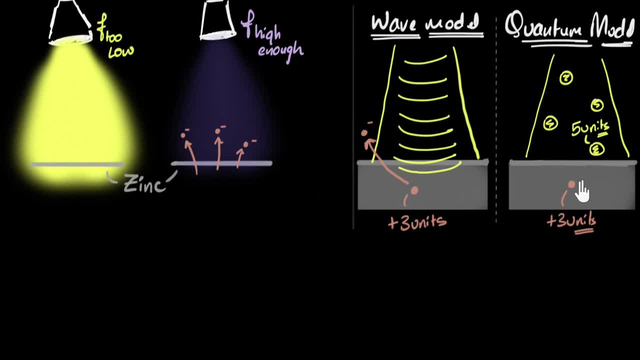 10 kilometers per hour, 20 kilometers per hour, 30 kilometers- Can you imagine that Direct jump? You can't imagine that. You might think that's so weird, but that's what quantum mechanics is all about. That's what quantum is all about. 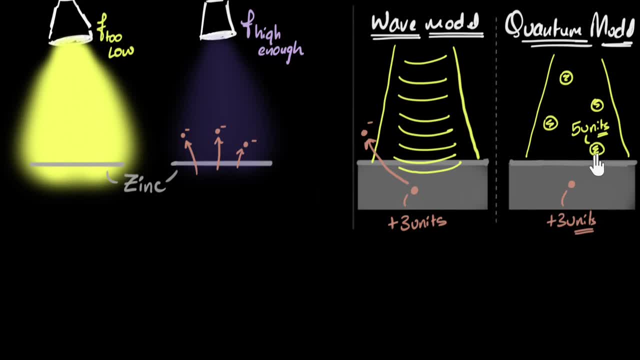 You can't get one or two units of energy. You either get all the five at once or you don't get anything at all. That's the weirdest, coolest thing about quantum mechanics. Anyways, once it absorbs that energy now, because it has gotten plus five instantly- 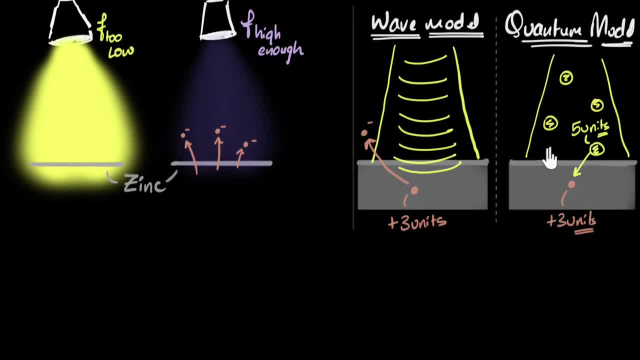 it has more than energy needed to escape, It immediately escapes and you get photoelectric effect. But now what if? what if the photon that we are incidenting does not have five units of energy? it has say, only two units of energy. 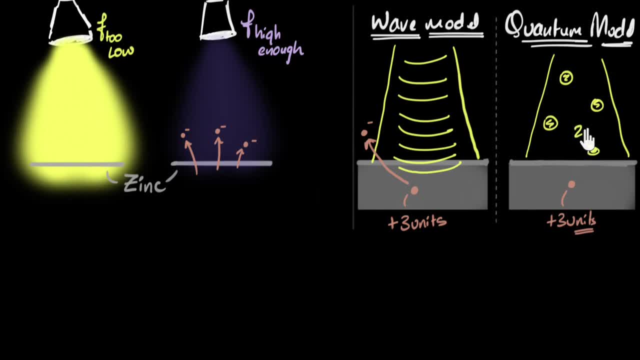 Let me draw a smaller photon to represent that. Okay, let's say it only has two units of energy. What would happen now? Now again, the electron would absorb that energy, but it's not enough to escape, And so it will still stay trapped inside the metal. 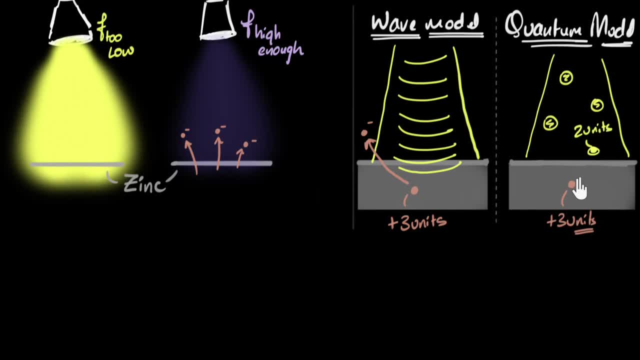 And so the electron does get excited because it has absorbed the photon of energy, But almost instantly it de-scides, It comes back to wherever it was before and, it you know, it releases that energy, Maybe in the form of, you know, heat, or maybe collisions. 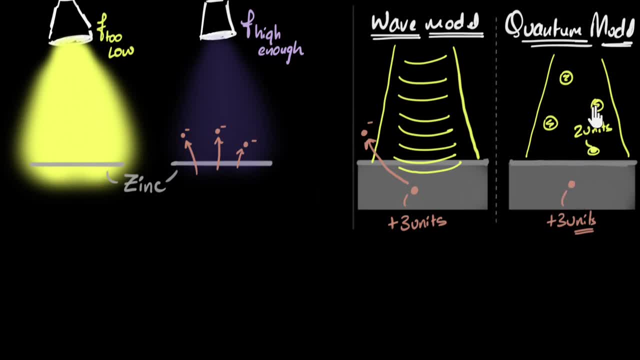 And so it comes back to where it was. And so now what happens if it obs, if it absorbs another photon? Same thing: It excites, then de-excites. Now, these electrons will always absorb one photon at a time. The chances of it absorbing? 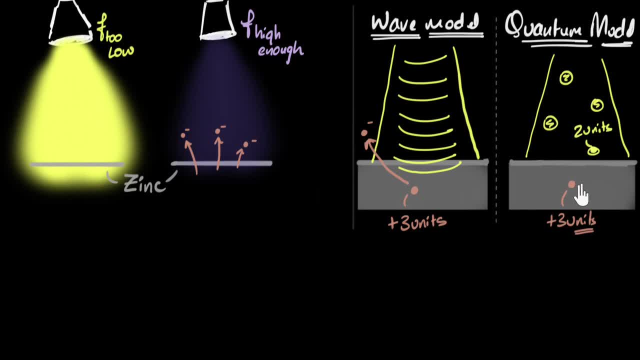 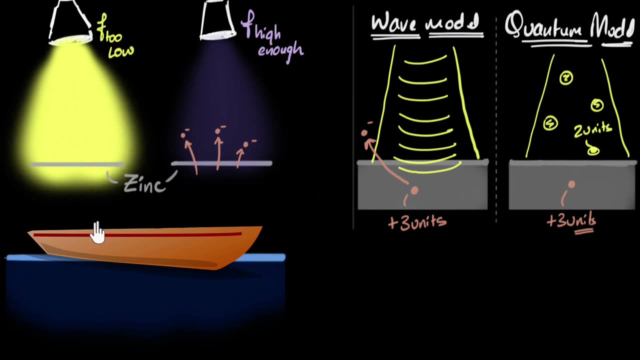 if it absorbing two photons at the same time is almost very negligible And therefore you can see, even if I shine millions of photons on this, it will not cause any photoelectric effect. It's kind of like trying to knock this boat out of the ocean by using ping pong balls. 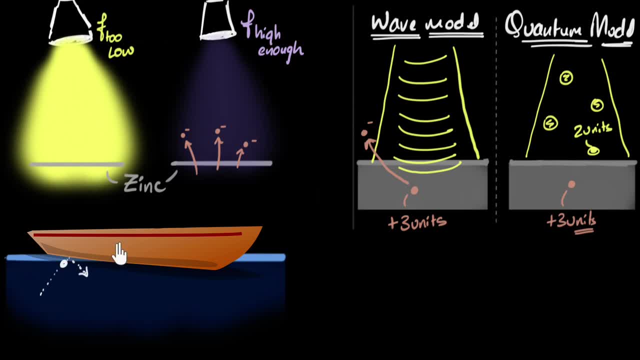 If you use a ping pong ball, one ping pong ball, nothing's gonna happen. So even if you shoot multiple ping pong balls, millions of ping pong balls, one after the other, nothing's gonna happen to this boat. The number of ping pong balls don't matter. 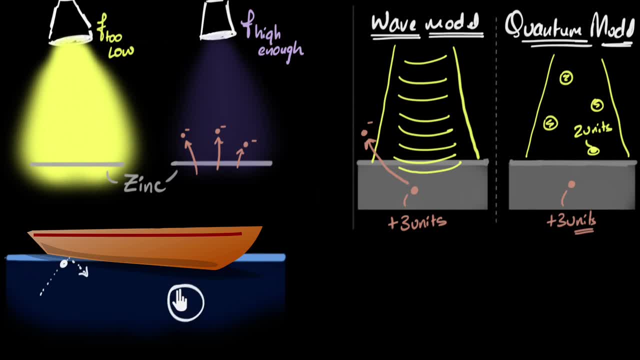 What matters is that a single ball. imagine you have a single large cannonball. One cannonball is all that it takes to shoot this boat and knock it off, And that's how you should think about it. The number of photons don't matter. 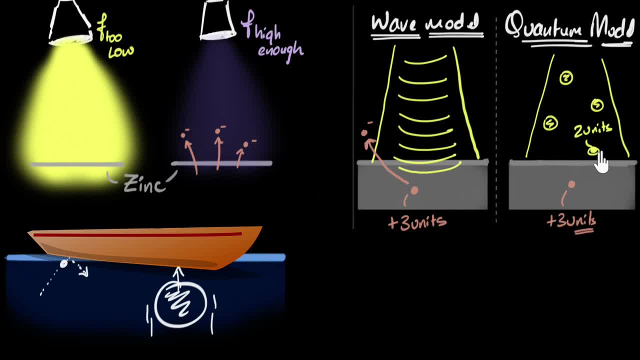 It's a single. a single photon should have enough energy to knock it off. Only then photoelectric effect will happen. And what does the energy of a photon depend on? You've seen the energy of any photon depends on from Planck's equation: 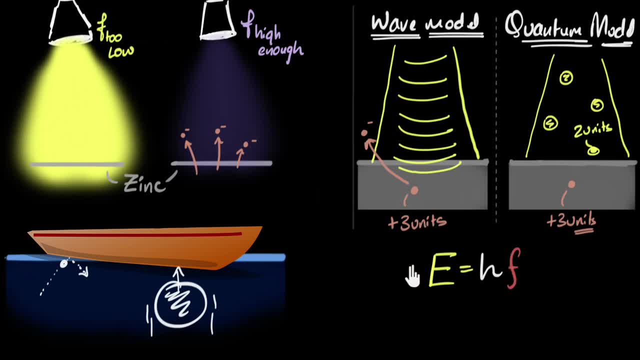 the Planck's constant H times the frequency of light. So more frequency of light, more energy of photon. So now can you pause the video and come back and explain why we don't see any photoelectric effect here, but we do see it over here. 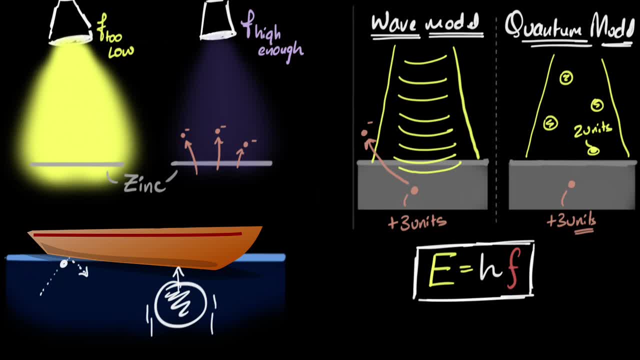 Pause and you can think about it. All right. so what might be happening over here? Well, because the frequency of the light is too low, that means the energy of the photon over here must also be too low, And so I'm gonna draw one tiny black dot. 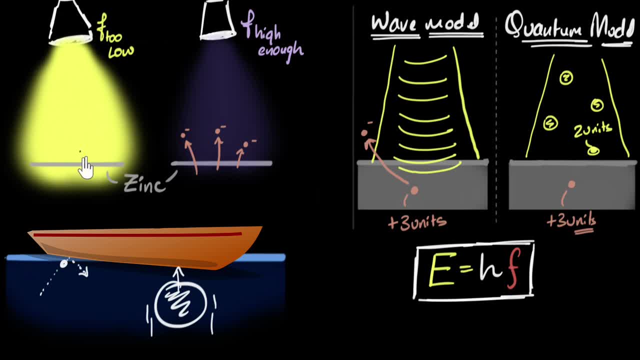 to represent very low energy photon, and it does not have enough energy to knock the electron off. That's why you get no photoelectric effect. But it's so bright. why doesn't that matter? Because brightness, high intensity means you have a lot of 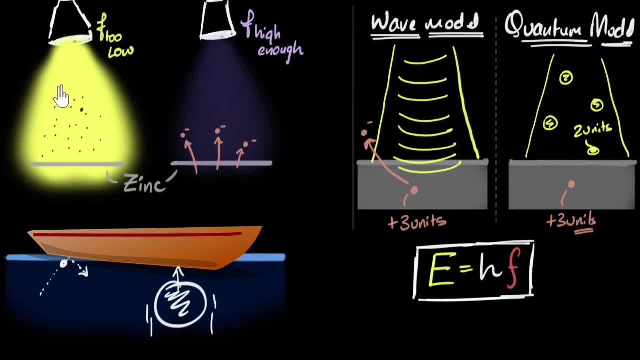 these photons, So let me draw lots of them. Okay, my pen slipped over here. So we have a lot of photons falling on a lot of electrons, but none of them have enough energy to knock them off, so you get no photoelectric effect. 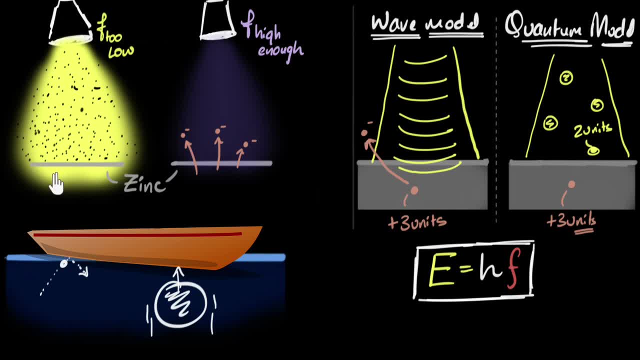 Like lots of ping pong balls coming and hitting this boat is not gonna happen. What's happening here? You have high frequency light and therefore the photon over here. I'm gonna draw a big photon over here. the photons have enough energy to knock the electrons off. 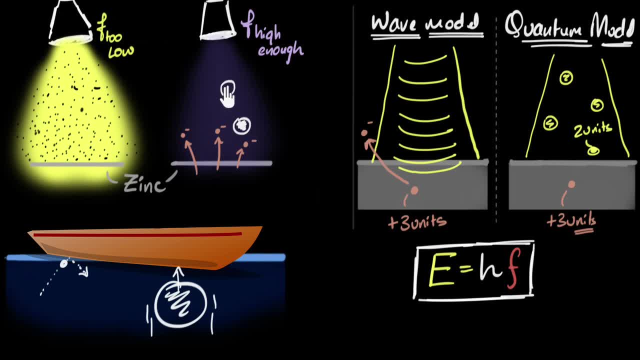 And so, but it's not gonna happen. It's so dim. So, yeah, it's very dim and therefore there might be very few photons over here- Very few. But whenever these photons get absorbed by the electrons, you get photoelectric effect. 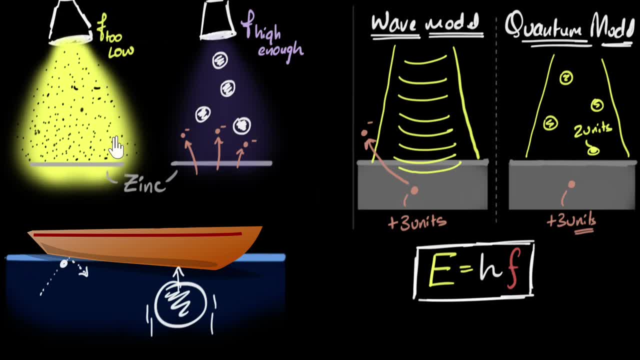 So you see what's happening. Even if you have a lot of energy over here, it's kind of like diluted into very tiny photons. None of them are able to do anything. And even if you have very weak energy over here, it's very concentrated into large photon packets. 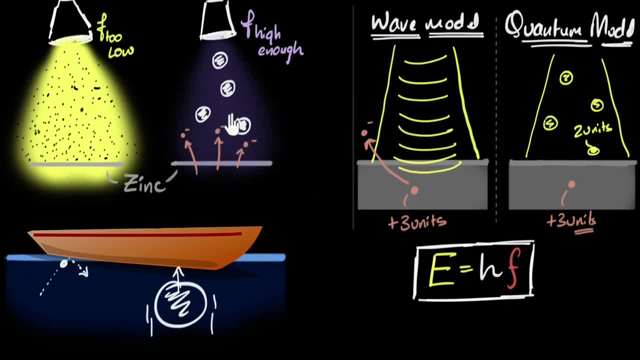 Each one of them is able to knock off the electrons, And that's why photoelectric effect depends on the frequency. Whether it's gonna happen or not depends on the frequency and not the intensity. Okay, but let's not stop here. Let's see if we can explain all the results. 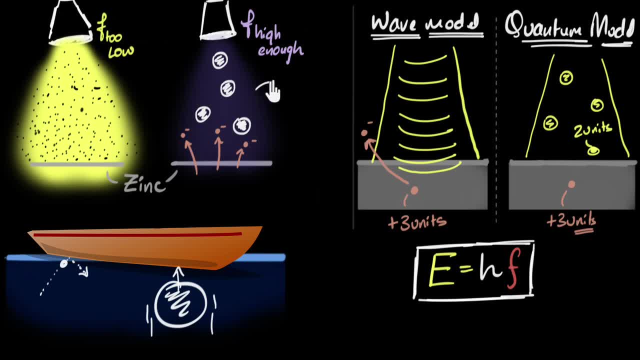 we saw of photoelectric experiment. One of the things that we saw is, even if you were to increase the intensity of this light, you make it more energetic. the electrons do not come out with more energy. We saw that the kinetic energy does not increase. 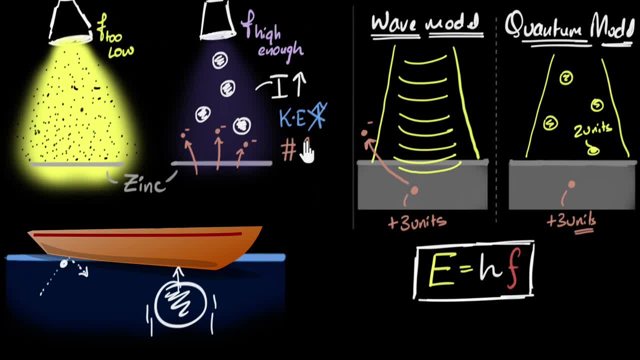 Instead, we get more energy. We get more photoelectrons- Oh sorry, we get more electrons coming out. Can you explain why this is happening? Okay, When you increase the intensity, you do not change the energy of individual photons. 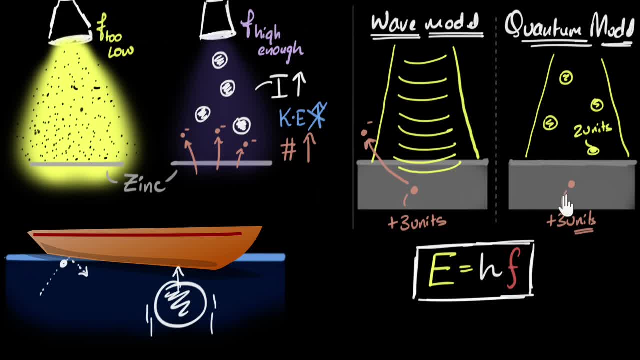 The energy of the individual photons stays the same, And therefore when an electron absorbs that photon, nothing has changed, And so the electron comes out with pretty much the same energy as before, And therefore the electron's energy does not change. But when you increase the intensity you do. 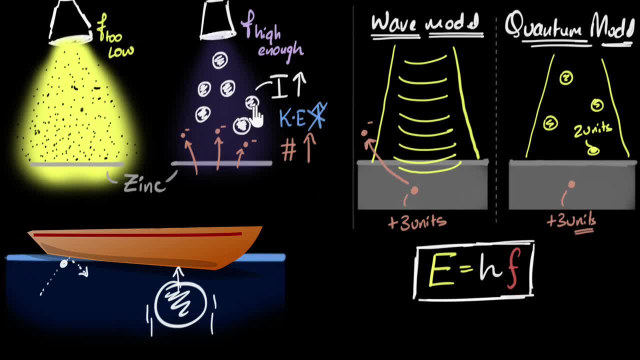 do increase the number of photons. So the number of photons increase And therefore now more electrons are gonna get those photons And therefore you expect more electrons to come out per second. So now it makes sense, Okay. The second thing we saw is: 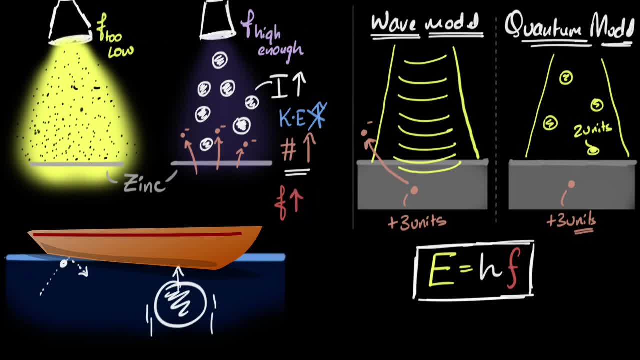 if you increase the frequency of the light, then the kinetic energy increases. Electrons now come out with more energy. Can you explain that using the quantum model? Yes, Because if you increase the frequency, the energy of the photons start increasing. Electrons gain more energy when they absorb that photon. 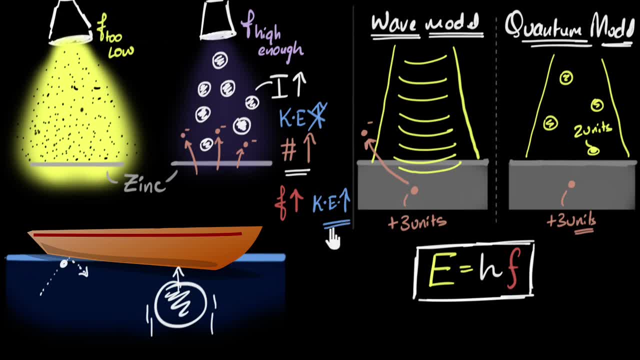 And so they come out with more energy. Now that makes sense. The final thing we saw over here was photoelectric effect is instantaneous, Even if you shine extremely dim light. as long as it's about threshold frequency, you get photoelectric effect instantly.